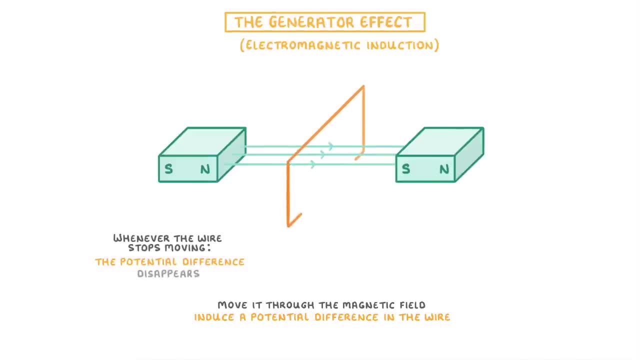 the bottom, then the potential difference disappears. This is because it's the change in the magnetic field that the wire experiences as it moves through it. The other thing to notice is that the direction of the potential difference swaps each time we change the direction, which is why the plus and minus signs keep switching around. 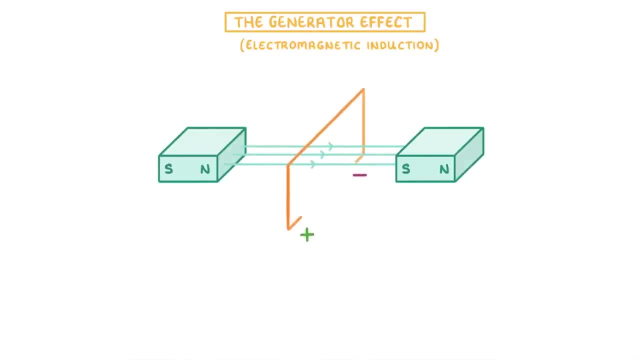 Now, at the moment, we just have a piece of wire, We don't have an actual circuit, And so, even though there's a potential difference, it can't generate any current. However, if we joined the two ends together so that we had a complete circuit, then the induced potential 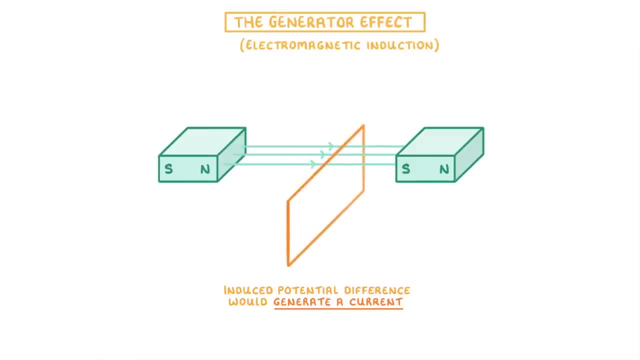 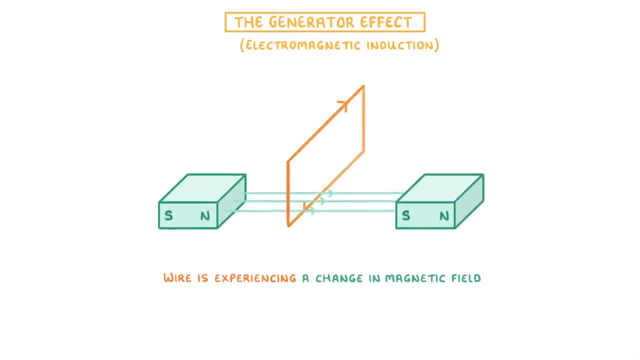 difference would generate a current, because electrons would be able to flow around the circuit. The same thing happens if we keep the wire still and instead move the magnets up and down. This is because the wire is still moving, experiencing a change in the magnetic field which, remember, is the key idea in electromagnetic 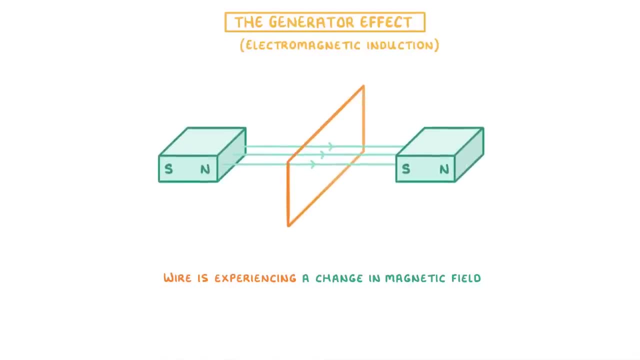 induction. If we instead move the wire back and forth like this, though, then this time there won't be any induced potential difference or current, because the wire isn't actually experiencing a change in the magnetic field. Now, if we wanted to change the size of the induced potential difference, and therefore 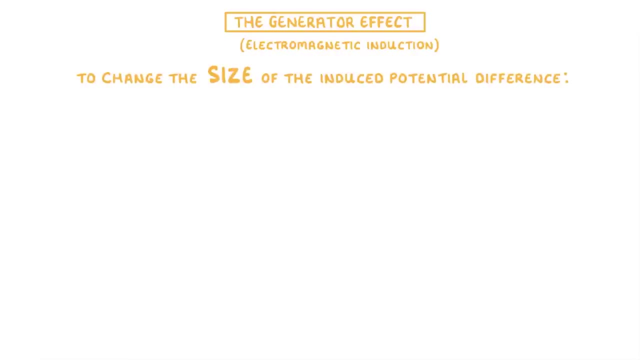 the current that it generates. we can do three things. One is to change the strength of the magnetic field. For example, if we used stronger magnets which produced a stronger magnetic field, then we'd induce a larger potential difference. The second is to move the wire or the magnets more quickly. 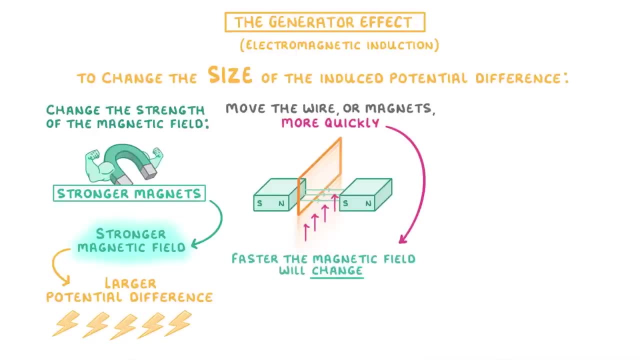 The faster they move. the faster they move, The faster the magnetic field will change, and so the bigger the potential difference will be. The final change we can make is to shape the wire into a proper coil so that it has multiple turns.